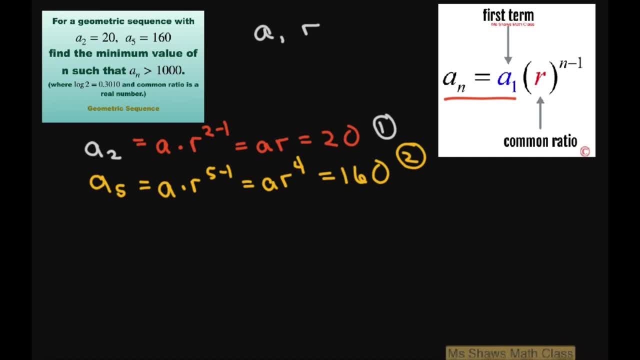 common ratio you take- let's see 2, and we're going to divide by 1, right to get your common ratio. So to do that, we're taking our second equation, which is a to the power of 4r, divide it by. 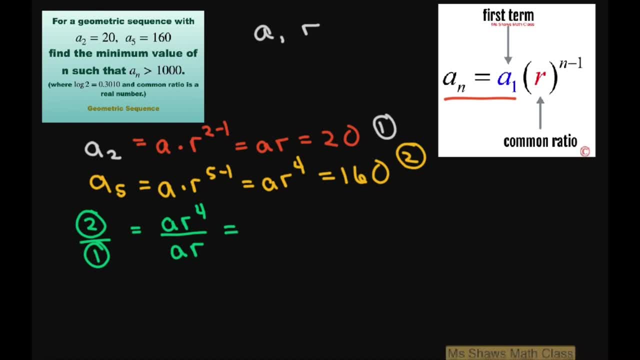 your first equation, which is a r, and that's going to equal 160 divided by 20.. Basically, what you get is you get the a's cancel here, so you get r cubed equals 8.. Therefore, r equals 2 cubed. 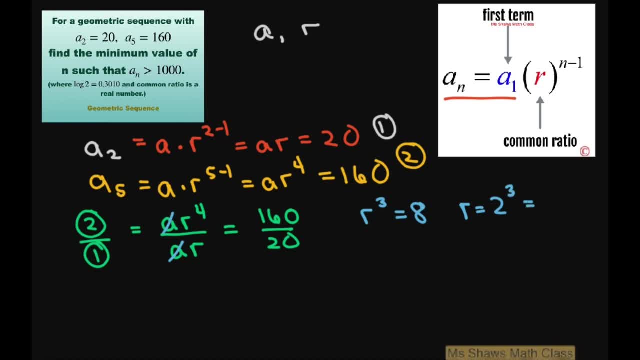 which is going to be a times r to the power of 4r, R is 2.. Because if we have r cubed, so r cubed is 2 cubed, then r is 2.. All right now, if my r is 2, then if I substitute it back into one of these equations, say this: 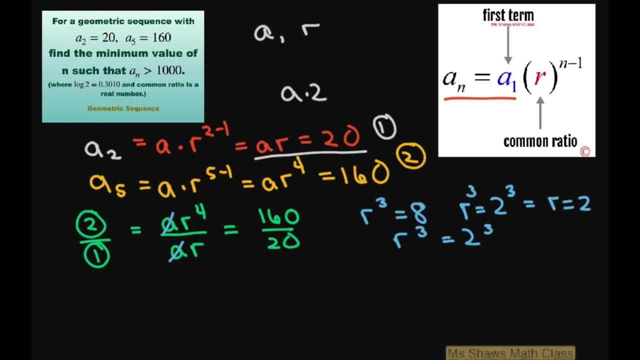 one I get. a times 2 equals 20.. That means my a equals 10.. So your first term is 10.. and your R is 2. now let's find our nth term. so your nth term is going to be your first term. times R to the power of n minus 1, and that's just filling out. 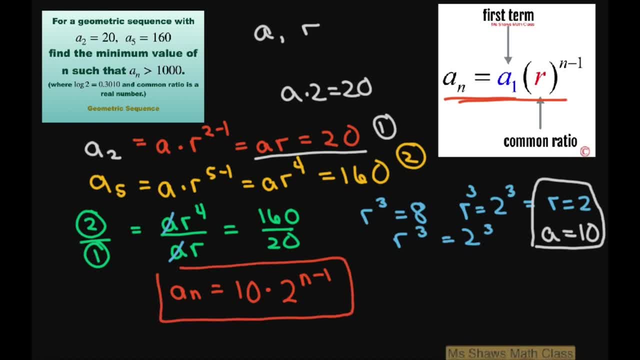 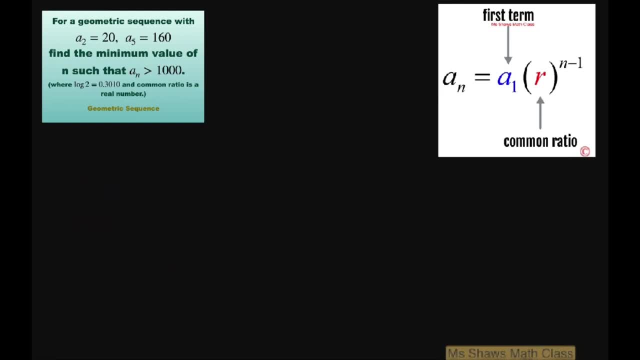 this formula. okay. so basically we want this to be greater than a thousand, and then we're going to use this information given. so we have 10 times times 2 to the power of n minus 1 is greater than a thousand. all right now. if you divide both slides by 10, we get 2 to the power of 2 in minus 1 is greater. 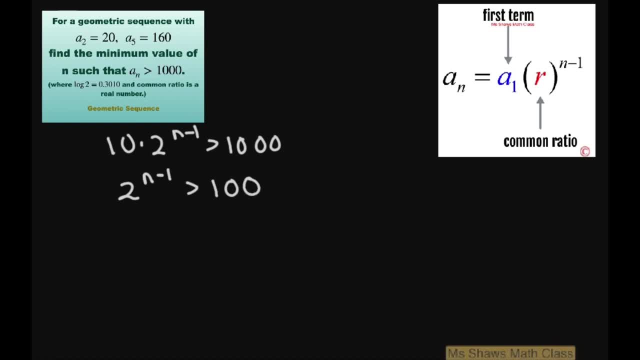 than 100. okay, let's take logs of both sides. you get log log. log of 2 to the power of n minus 1 is greater than log of 100. all right, so we can rewrite this using your prop power property of logs. this is going to be log.